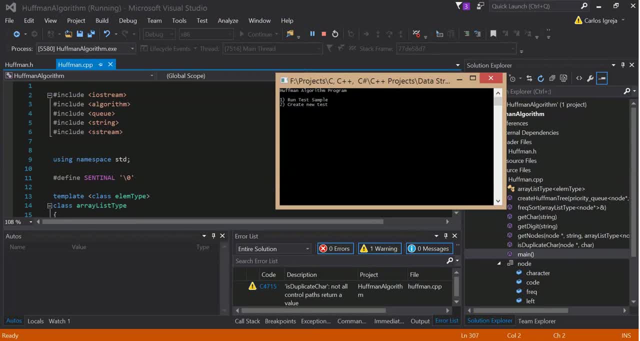 Hello, my name is Kalsik Rajan. This is a C++ project that I did for data structures and algorithms. This is the Huffman algorithm. I'm going to run a simple test And there it is. So: characters, frequency and the code. So the highest frequency of the character should have the lowest code, The shortest path. So that's the idea And basically, I'm going to run a simple test. 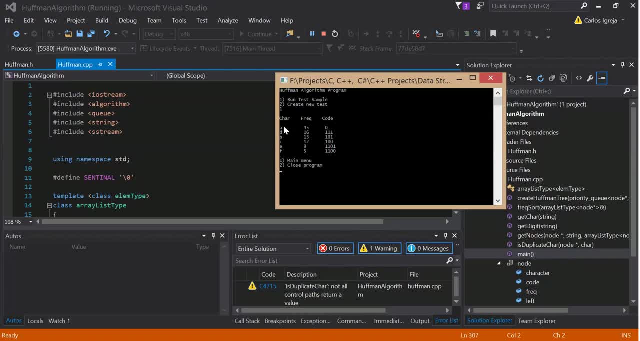 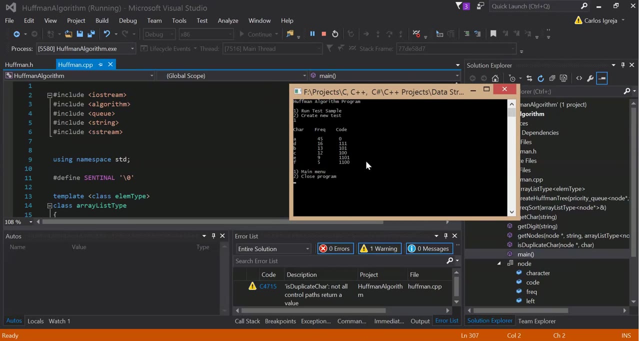 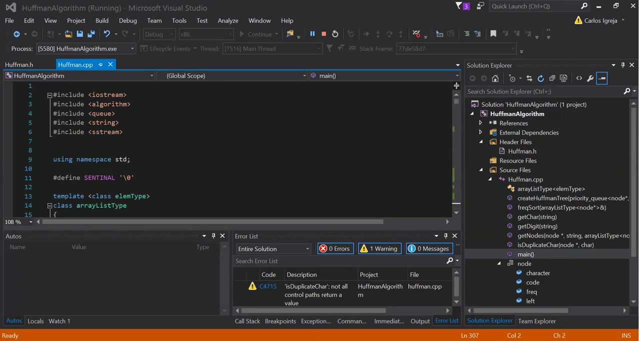 The characters might appear And basically the frequency that they occur, And then it just so it's stored this way And that's the idea of the Huffman algorithm. So yeah, that's pretty much it. I don't think it needs any more explanation, But I do have this, the wiki, And you can see. 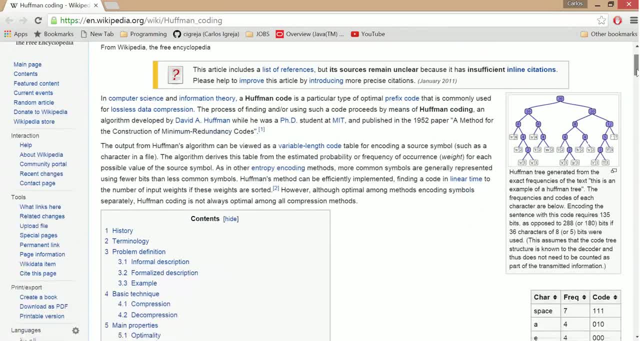 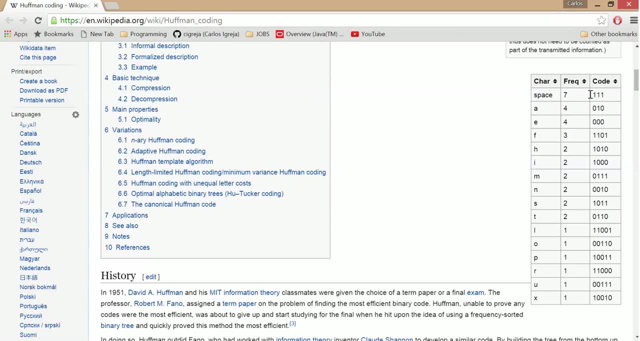 the tree basically looks like it has nodes And that's the Huffman tree And you can see it has a code, And the highest code- I mean the highest frequency for that given character- should have the smallest code or shortest path, And yeah, so that's basically what my application does And I'm going to. I'll go over the code now. 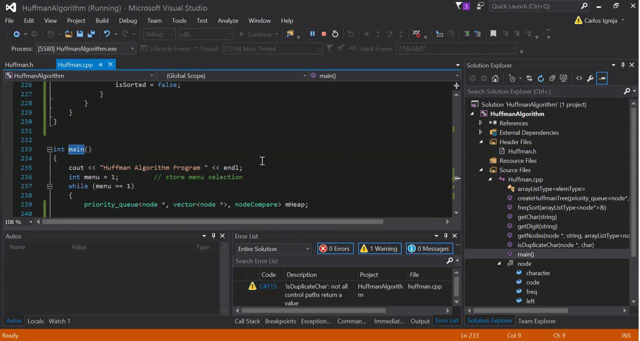 So this is the see-out, This is the main, So I'm going to go over the main. And it uses a priority queue, Takes the node pointer vector of node pointers, node compare, and this is the M heap. So just a lot of you know the GUI, the see-out stuff. 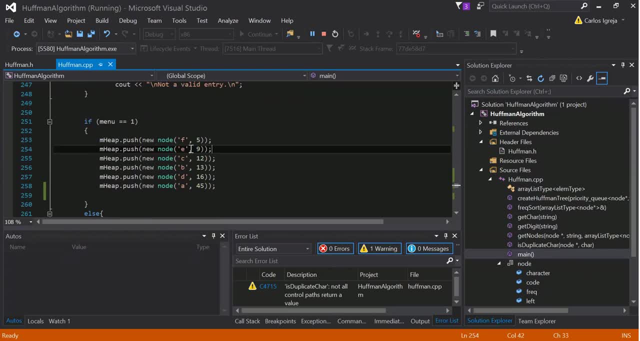 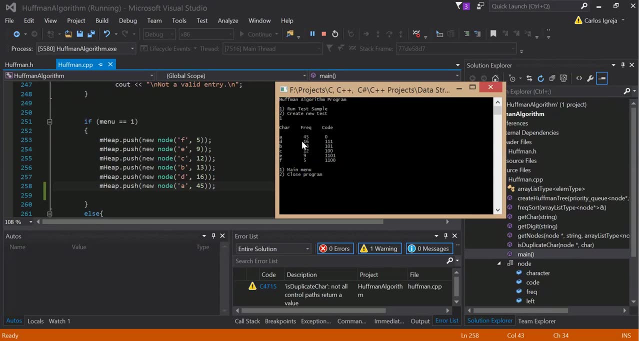 So obviously I used. this is what I used for the test. I did it in reverse order And then you saw that it was in reverse order. So this is the see-out stuff. So this is the see-out stuff was an output. as you can see, it gets outputs with the highest frequency and 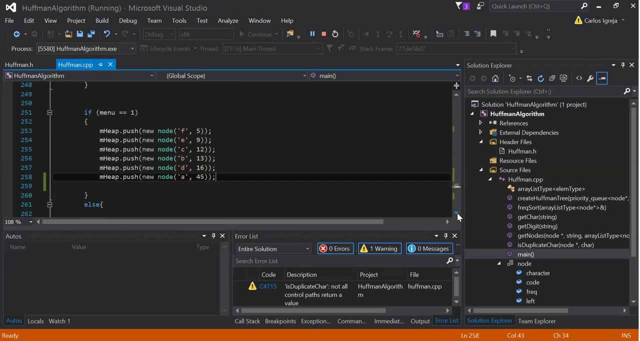 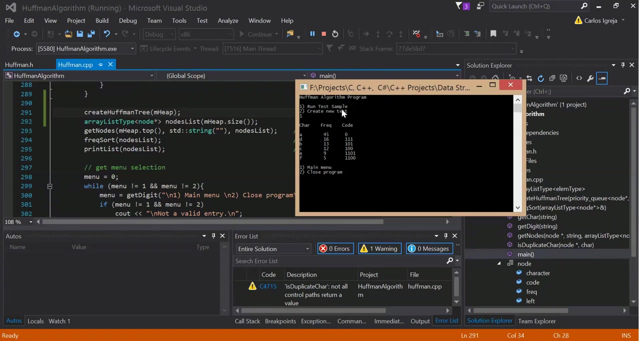 displays like that. so so AC is a character and the frequency. so this is when, if I chose not to use it, the test sample- I can enter the character and frequency for each node. it will create and add that and make my own. so yeah, right here. so you see, if I choose one, I can run test sample. if I chose two, I 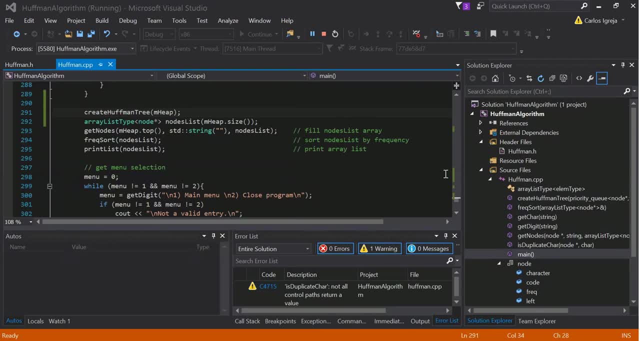 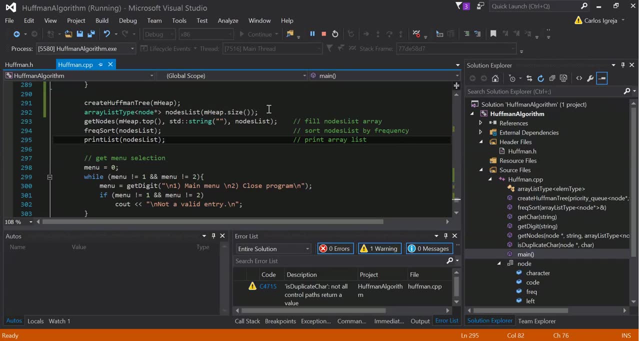 could create. just create my own random test. but the test sample is my ideal for this demonstration. create Huffman tree. so this is going to create the Huffman tree. then we're going to declare a node list, just an array of node pointers. it's going to be the size of the heap and get. 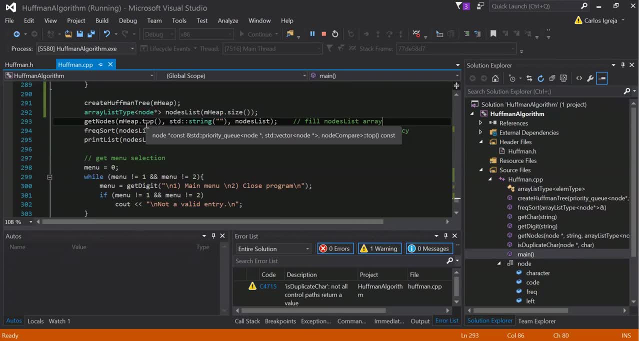 nodes past the M heap top, it will. this is the path. so we're just going to first pass the empty path and node list, which is the array here that we just created, and then I'll do the frequency sort. so basically this is just source, the source by frequency, and then 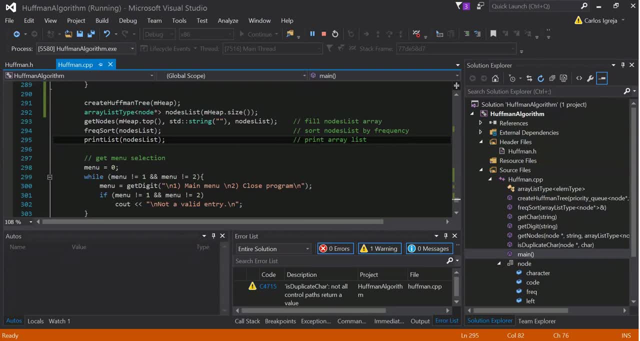 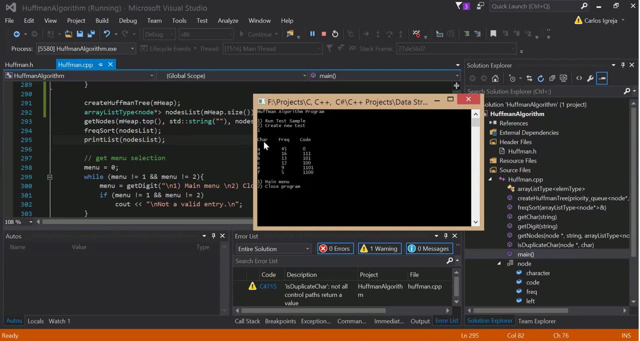 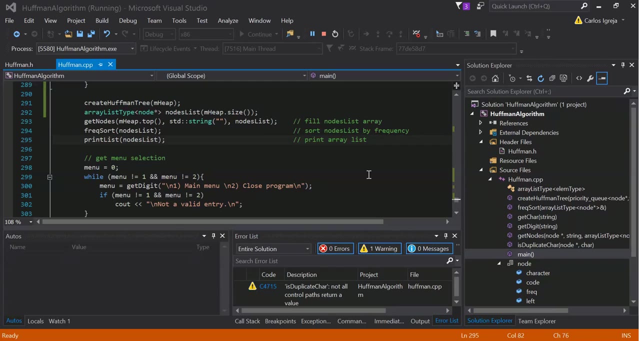 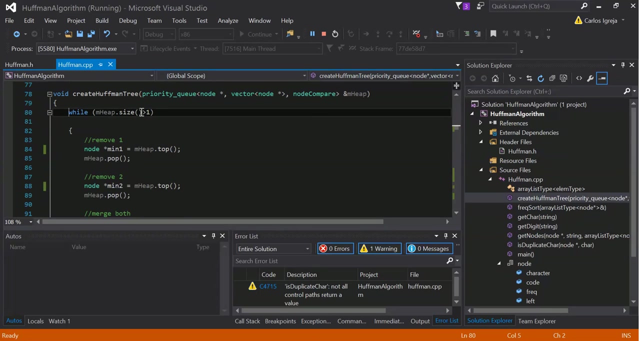 this just prints out of the, the, basically the output data to the screen, to the console. so we'll output this header and just all this information for each node, and so I'll go over each one of these now. so the create Huffman tree takes a the M heap. this is a while loop M heap until M. 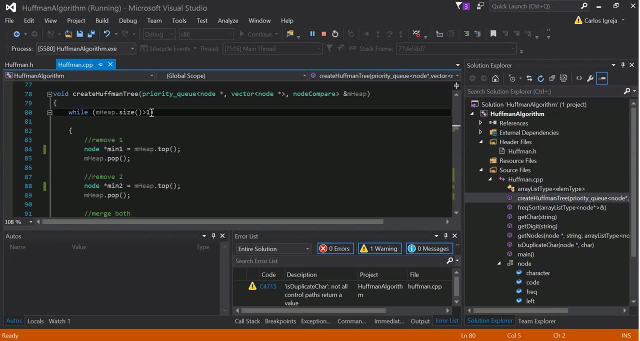 heap is greater than one, as long as M heap is greater than one. so this is remove one, remove two and then merge both. so min-1 just takes the value of the top value of the heap and then we pop it so it removes it from the. 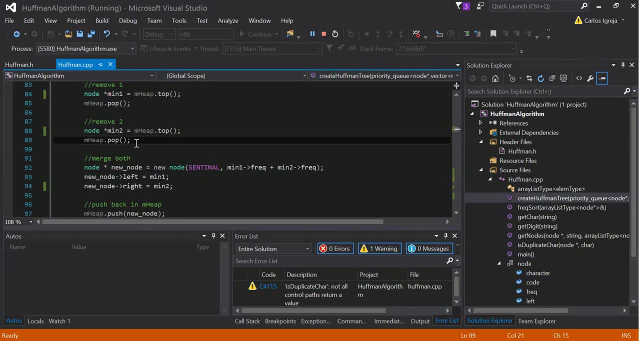 heap same here for the second one. we get the next one and then remove that. then we create a new node and we take the two frequencies, add them and then- and senton is the, I guess, the car, and this is the frequency of the new node, the car sent. 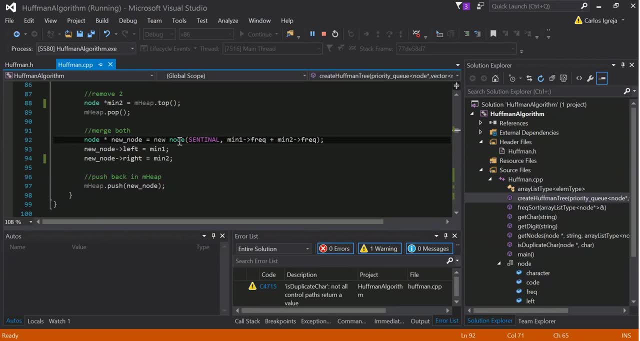 to know. this just means don't include it. this node is not included. and store, and that new node to the left will store the first one and then to the right will store the second, second, one, basically, and one and two for a second. the same difference really. and there's just two nodes: push back and M heap, so put the. 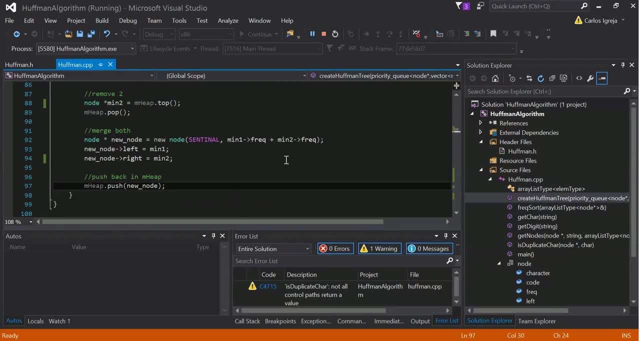 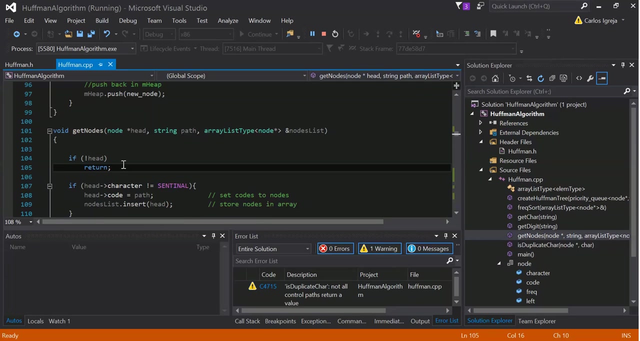 new node and the heap and then that's all this does. next is the get nodes. this takes a node head point to a string path and the node list cannot head. so that returns head character not equal a sentinel. so, like I was saying, something will not be. 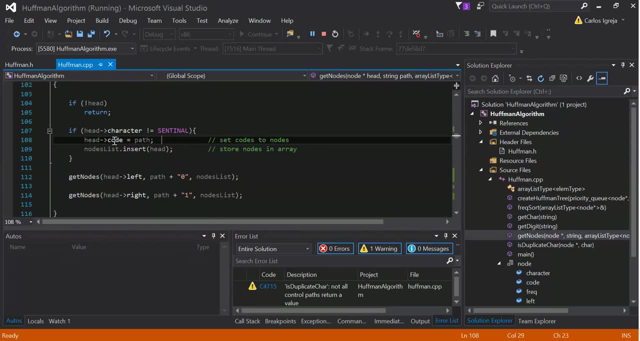 included. so other than that, the head cold will equal path and the no list enter head. so yeah, and then what happens here is get nodes will pass the head here and get the left and it will add the path plus 0 or path plus 1 for the right, and that's essentially all it does, just yep. 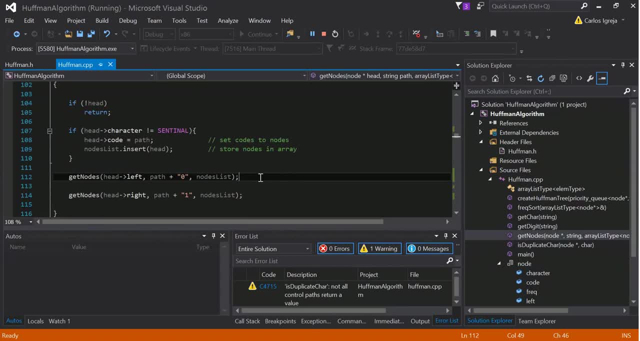 calls this method recursion and that's it. so that's how we get the paths and basically, as you can see, we'll build a tree. it will all across, so that is 0, 1, 0, 1, all the way across, and then just keep doing that but ignores the Sentinel. so, as you can see, the codes are are pretty.